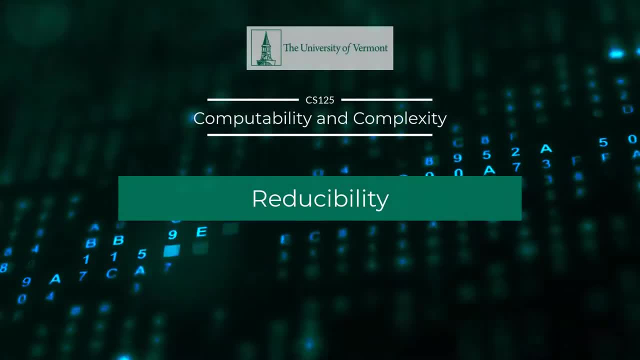 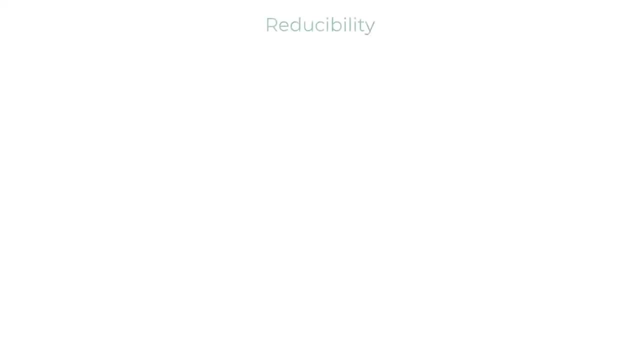 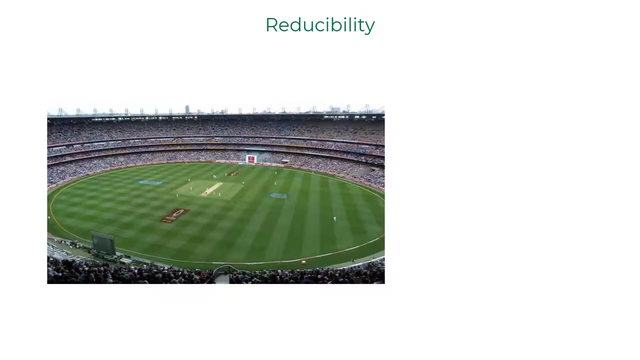 Let me start this lecture by describing the concept of reducibility with an example. Here is a playground that is circular and you would like to calculate the circumference of it. How do you measure the circumference? Should we look for giant circular scales or do we have a better? 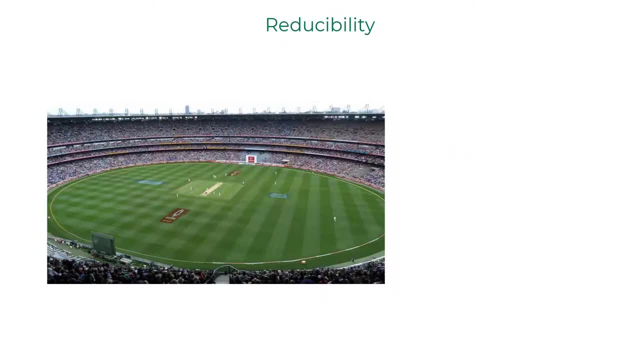 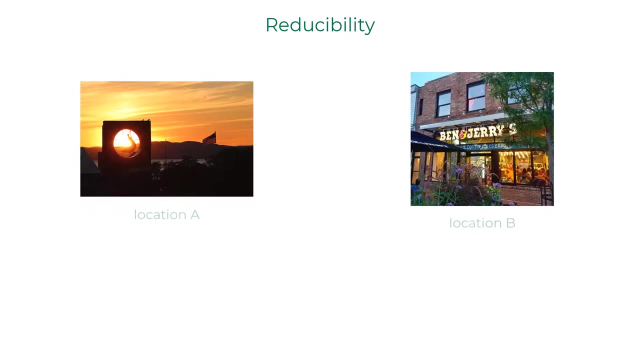 solution. The problem of finding circumference of a circle reduces to the problem of measuring the radius of the circle. With just a small scale and a medium-sized rope you can solve this problem. Here is another example: The problem of walking from location A to an unknown location B in a city. It reduces to finding the directions. 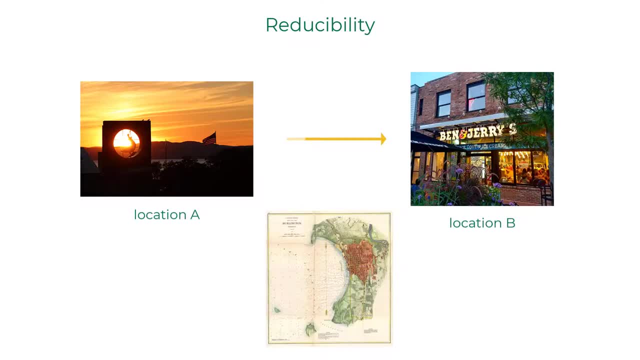 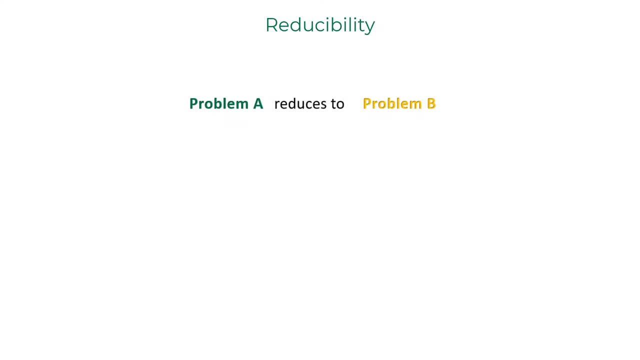 on a map for that city. Now let's say A and B are two problems and problem A is reduced to problem B, Meaning if we solve B we solve A as well. In the context of theory of computation, if A is a threaten of A, then A is a preventing option A of B, which means if B is a looking tone B. so all A and B are positive examples of C. If A is a erase noble, then so are C and B and B In the same context. if C and B are positive, then A and B are. proposal A- The definition of time irregularА is a try to compare A and B from M to B and B to M. 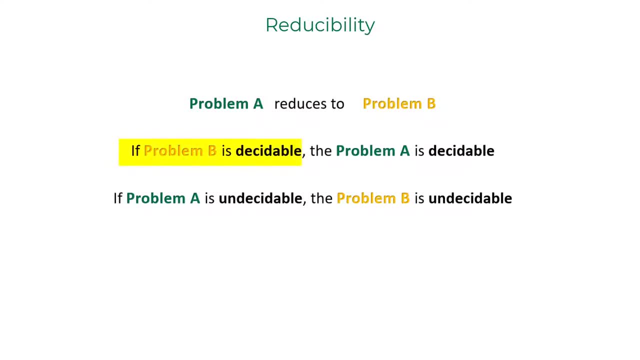 A can be reduced to B and B is decidable, then A is decidable. If A is already known to be an undecidable problem and is reducible to B, then B should also be undecidable. Let us consider the problem of traveling from our galaxy to the neighboring galaxy overnight. 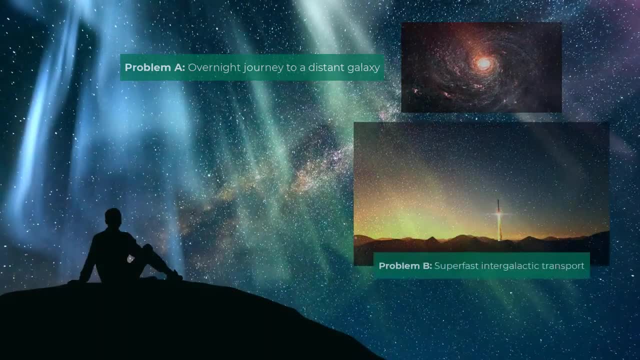 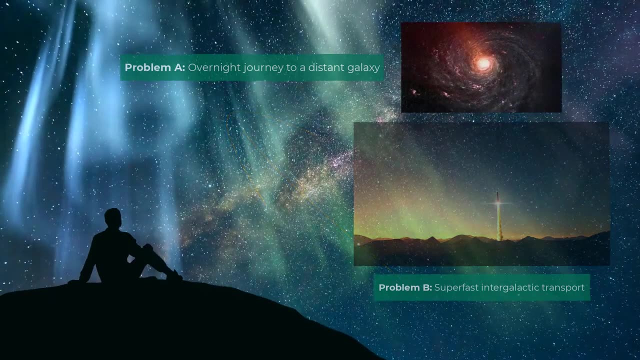 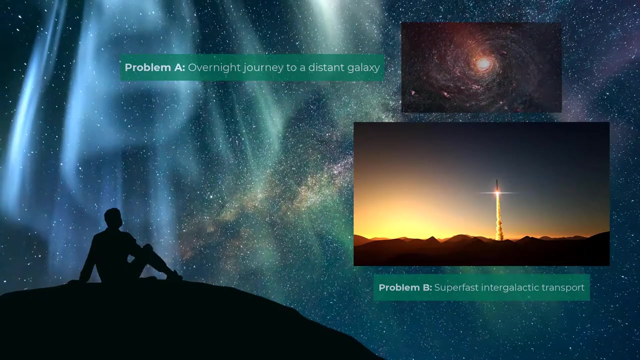 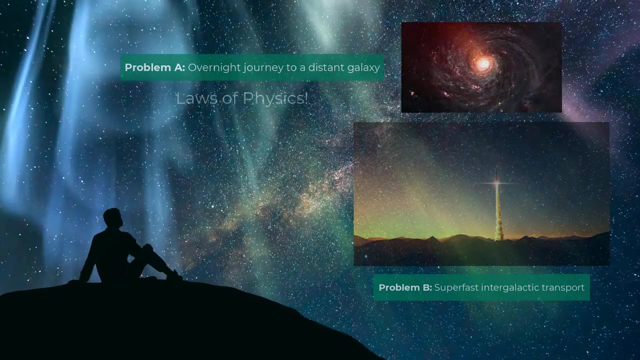 We shall name this problem A. This problem reduces us to the problem of building an intergalactic spaceship that can safely transport us overnight. Let's call this problem B. The closest galaxy is 2.5 million light years away, meaning it will take us 2.5 million years if we travel at the speed of light. hence, problem A is. 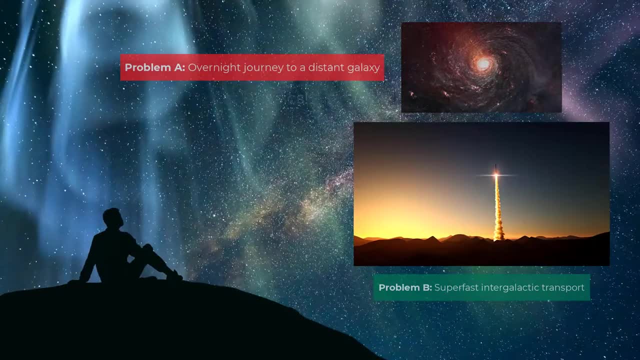 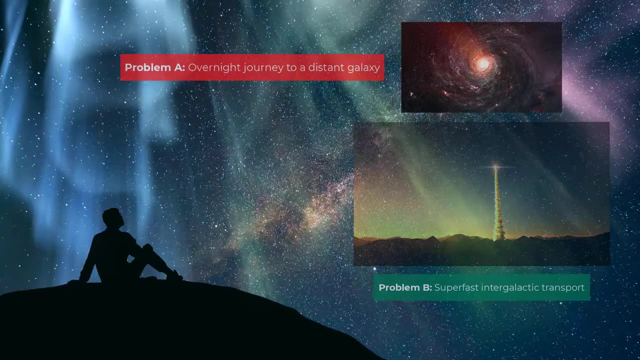 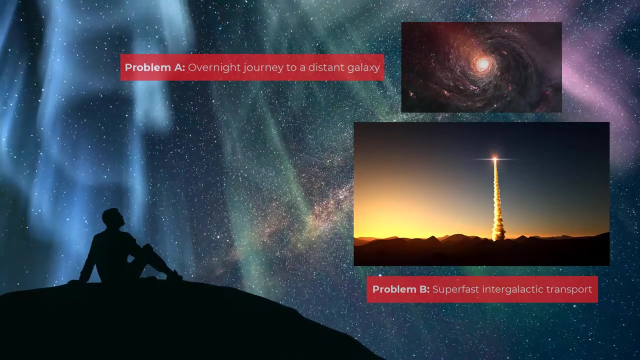 unsolvable, But problem A reduces to problem B, meaning if a solution exists for problem B, then a solution exists for problem A, which gives rise to a contradiction, as we just proved. problem A is unsolvable, Therefore problem B is unsolvable. 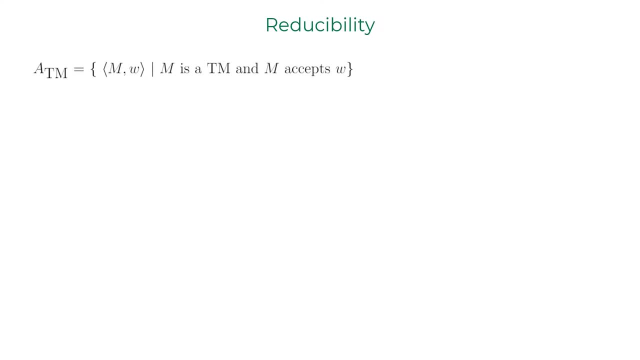 The same logic can be applied for proving undecidability of certain languages that the language ATM. the acceptance problem of a Turing machine is undecidable using diagonalization technique. a decider for ATM does not exist. Now let's say a decider for: 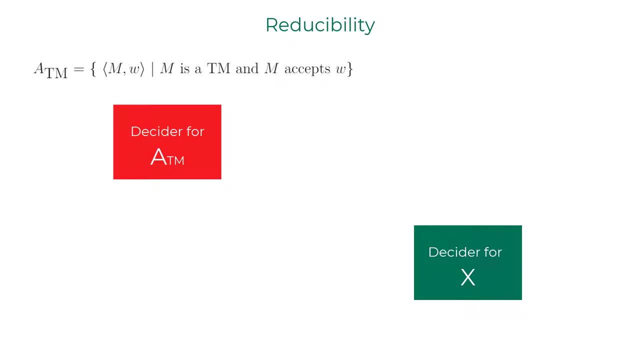 a certain language X somehow decides the language of ATM, which is already proved to be undecidable, Then we can confidently say that the decider for language X should never exist and the language X is undecidable. Okay, so using the same logic, I would be proving to you formally that halting 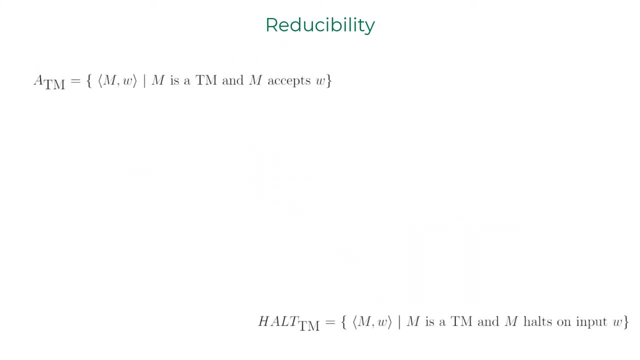 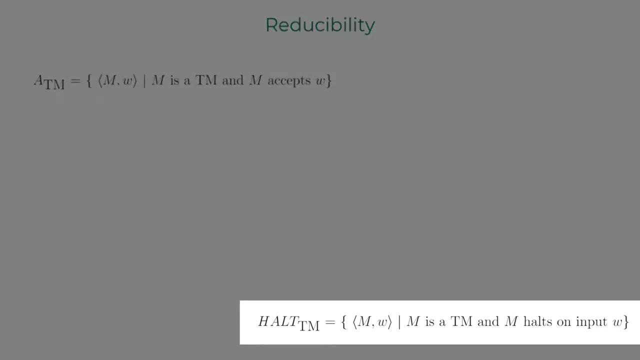 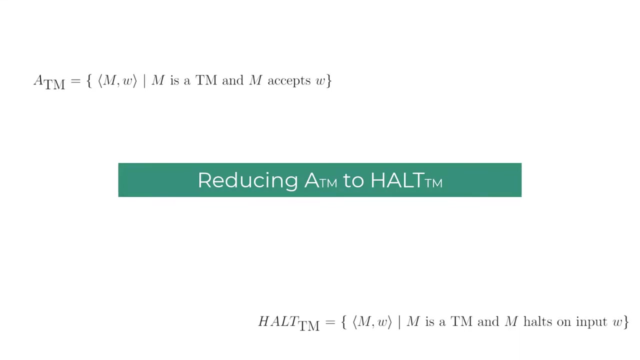 problem is undecidable. Let us consider the language HALT-TM, Defined formally this way: it consists of strings that contain the pair Turing machine description M, and the strings for which the machine M, halts. Using the technique of proof by contradiction, we shall prove that HALT-TM is undecidable. 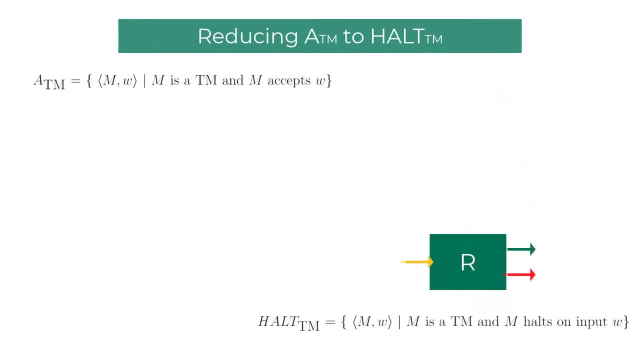 So the first step is to assume that a decider exists for HALT-TM. Can we use this magic decider box of HALT-TM to build a decider for ATM? Time 2 Turns out we can. Here is the formal proof. I will try to explain it to you as well. 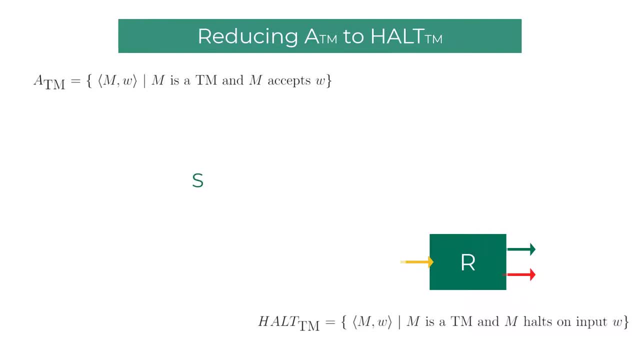 Time 3. Tip 1: We can build a decider for ATM by using a magical decider R that decides HALT-TM's argument. Turing MachineỐ S. Tip 2: We will simulate machine M on string your name. Press Enter to open your Notepad. Now the machine is not working. You must stereotype yourU рассказ out loud. 2: We see that the machine does the same for Either of the patterns. It is not machined by μαςuting TypeW and using String W without 땅의 데이 Maß in. 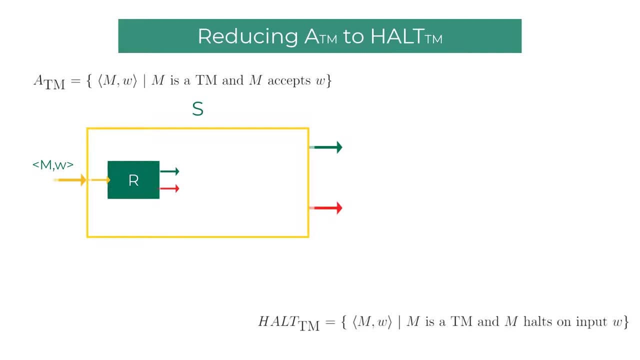 On HALT explains a problem which brokers usually Carm O енным or the not. That is the absolute key for all options or occasions to burnt on HARTTM. decider R. If R ends up in reject state, it means the machine M will end up. 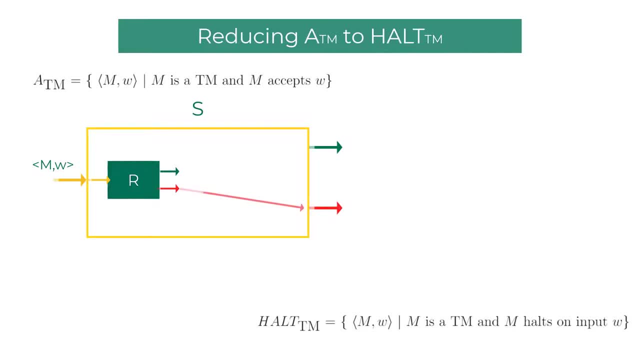 in a loop on string W. Hence there is no way machine M is going to accept the string W. So the decider S, which is supposed to decide ATM confidently, can reject the machine string pair M W. Perfect, So I've drawn the circuitry that's going to do that in that. 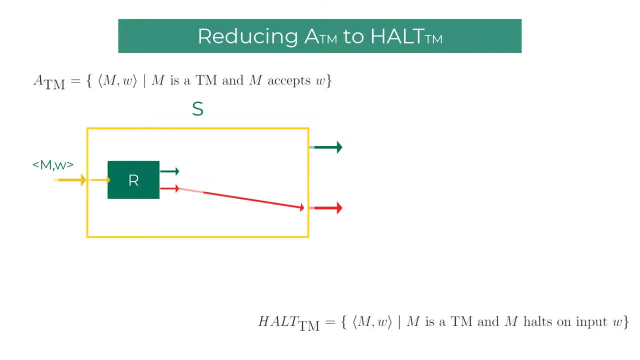 machine. All right, When HARTTM decider R ends up in accept state, it means that the machine M will halt on input string W, But it does not say whether it halts on an accept state or a reject state In the machine M. Okay, So all it says is that the machine M halts on the input string. 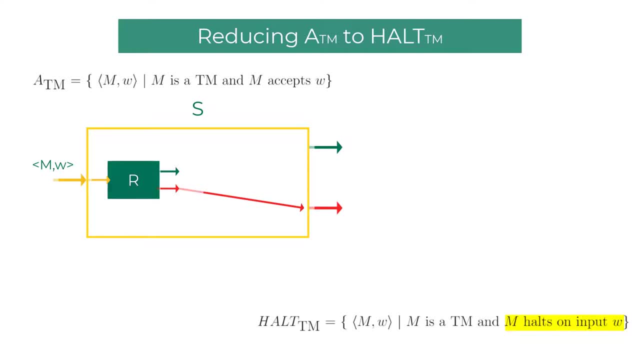 W. So what do we do now? What we can do is confidently simulate M on W on a universal Turing machine and see if M ends up in accept state or a reject state. There is no way this universal Turing machine will end up in a loop. 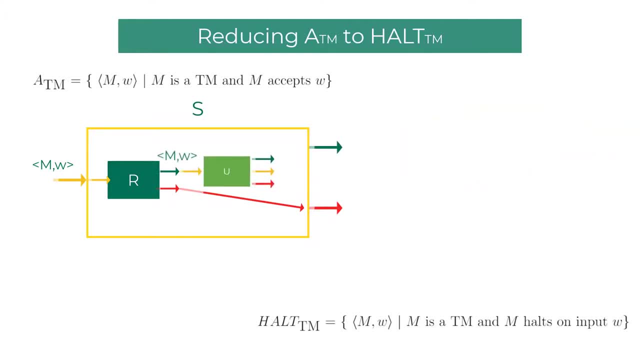 Because HARTTM decider R just certified it will halt for surely on input W. So if the machine M ends up in accept state on string W, make sure S ends up in the accept state. If the machine M ends up in reject state, make sure S ends up in reject state. So there, 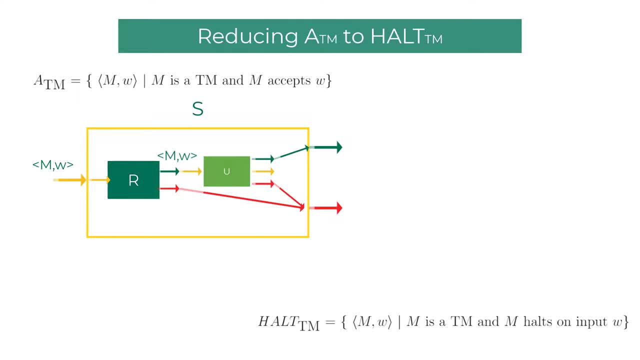 you go. So I've connected the universal Turing machine that is simulating M on W. The connections for accept and reject state are going to the accept and reject state of the decider S. Hence we are able to build a decider S for ATM using decider R for HARTTM As no decider. 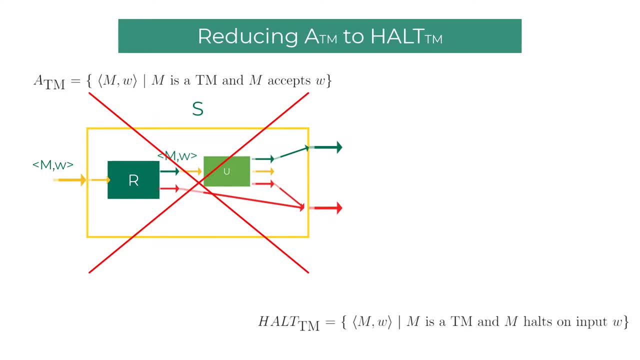 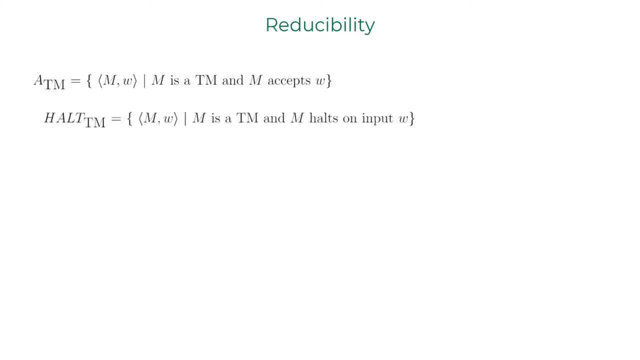 exists for ATM, the magic decider R for HARTTM does not exist in reality. Hence HARTTM is proved to be an undecidable language. Now we have two known undecidable languages and an uncountably infinite set of undecidable. 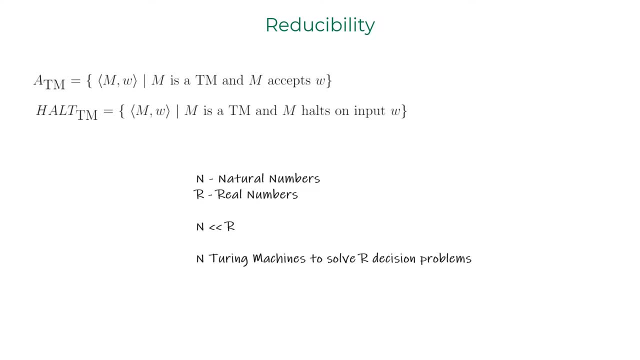 languages waiting to be discovered. You will be introduced to several languages later on that are proved to be undecidable using the same technique. When a problem A reduces to problem B, If problem B is decidable, then problem A is. if we already know that problem A is undecidable, that will imply a. 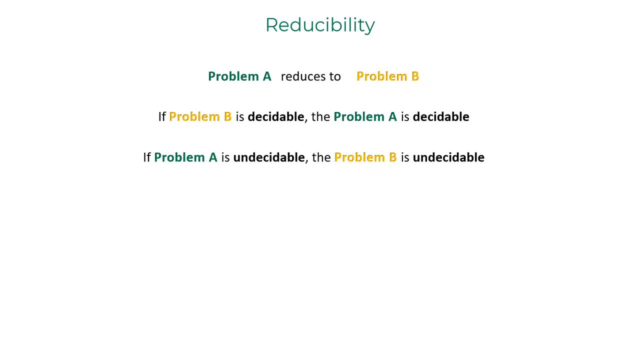 decider can never exist for B. hence B would be undecidable as well. I'll spend some time here explaining the logical fallacy new learners can fall to. Let's say the problem A reduces to the problem B. If B is unsolvable, it does not mean. 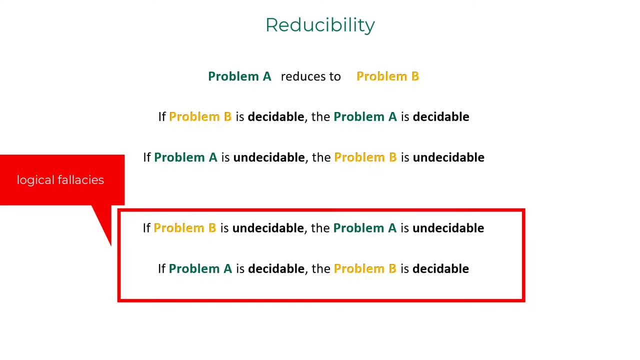 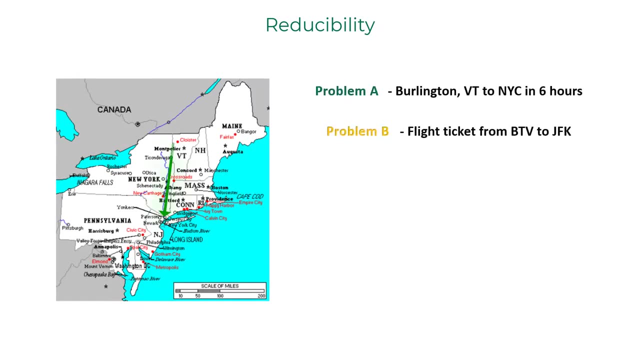 that A is unsolvable. The problem A can reduce to multiple problems. Even if one of the problems is solvable, then A will be solvable, right? The problem of traveling from Burlington to New York within six hours reduces to buying a ticket to the flight from BTV to JFK because it takes only about an hour and 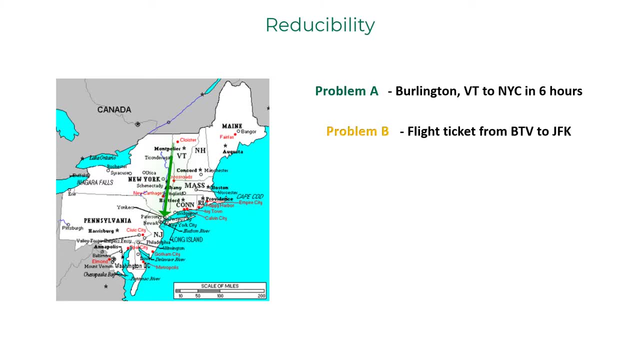 a half. Just because the flight gets cancelled does not mean that you cannot get to New York. from New York, You might as well drive. The other logical fallacy is that when A reduces to B and A is solvable, it does not mean B is solvable. Think about this example: The 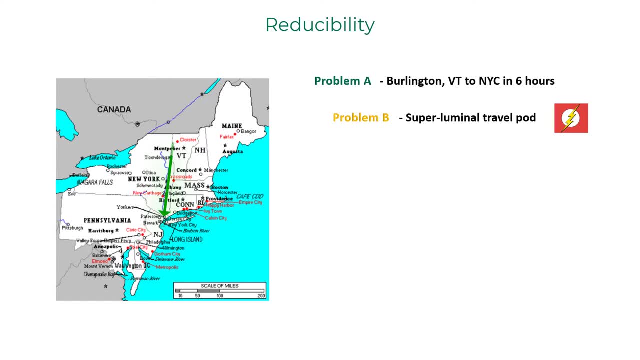 problem of going to New York to Burlington in six hours can also reduce to superluminal traveling pod, a vehicle that travels faster than speed of light. Just because you can get to NYC from Burlington within six hours does not mean that you have solved superluminal travel. okay, I will end this video by